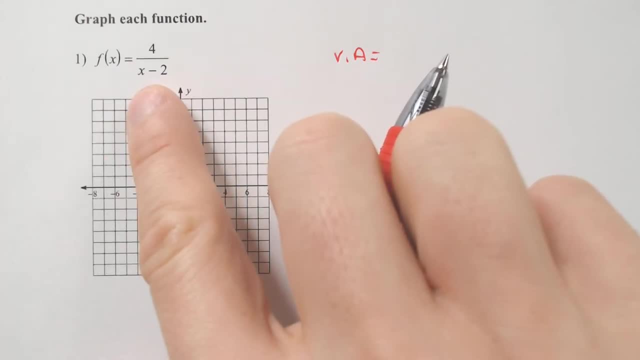 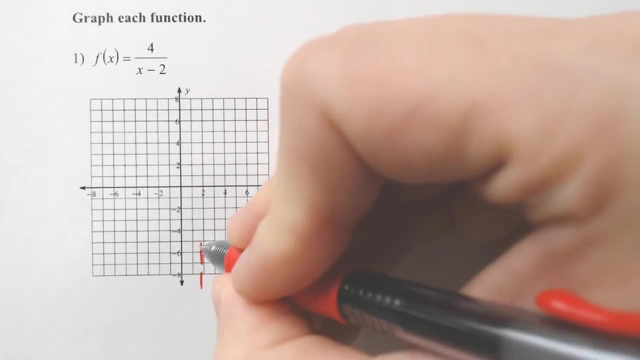 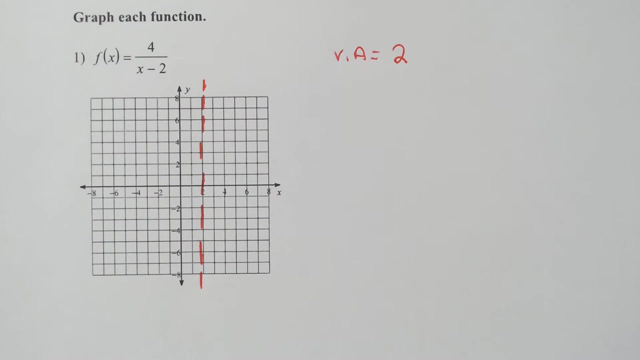 set the bottom of the fraction equal to zero. So if you set x minus two equal to zero, your vertical asymptote in this case would be regular two. So I'm going to draw a dotted line here at x equals two vertically, and then from here we would want to figure out what the horizontal 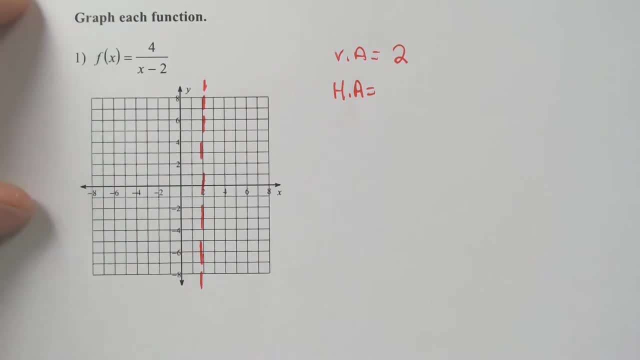 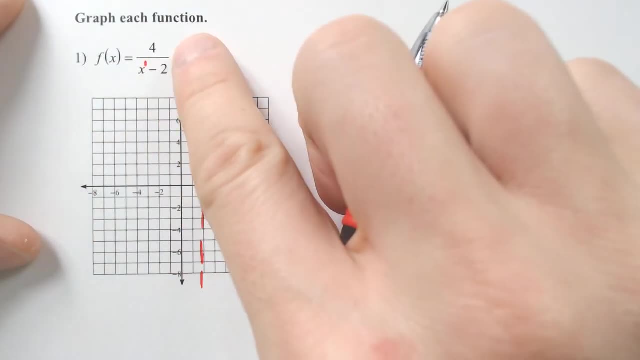 asymptote is Now. the horizontal asymptote is based off the exponent. So if it is a smaller exponent- which it is this time- over a bigger exponent, we have x to the first on the bottom. we have no x's on the top. that will guarantee the horizontal asymptote. 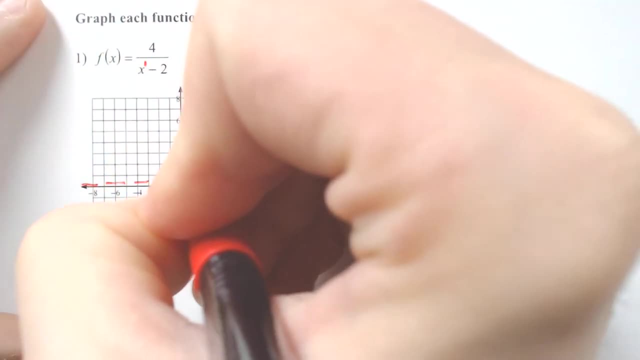 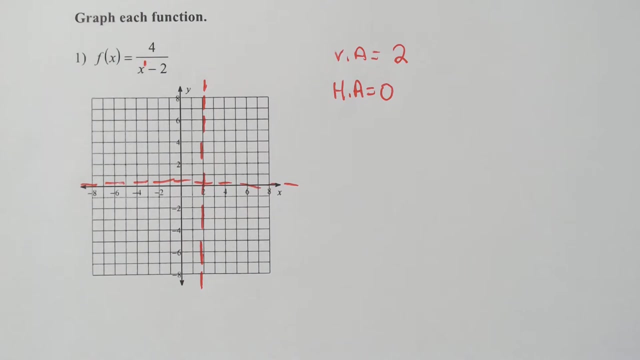 is equal to zero. So we're going to draw a dotted line here at x equals two vertically. The horizontal asymptote is zero, So we draw that dotted line there horizontally. The next thing that I would recommend doing is plug in any number for x that you want. However, I would make 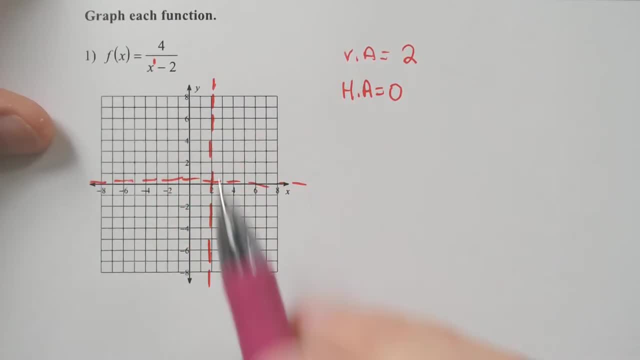 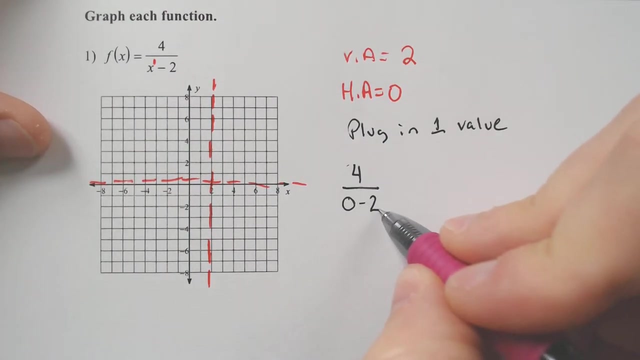 sure that it's kind of close to the vertical asymptote. But another good number is: always: plug in zero if you can. if you can, And if we do that, plug in one value, we would have four over. I'm plugging in zero, zero minus two, which ends up being four, over negative two, which is. 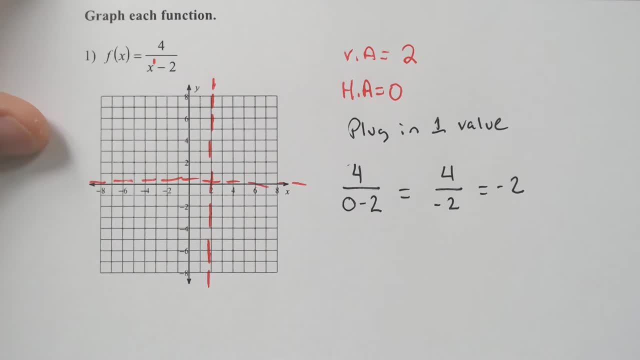 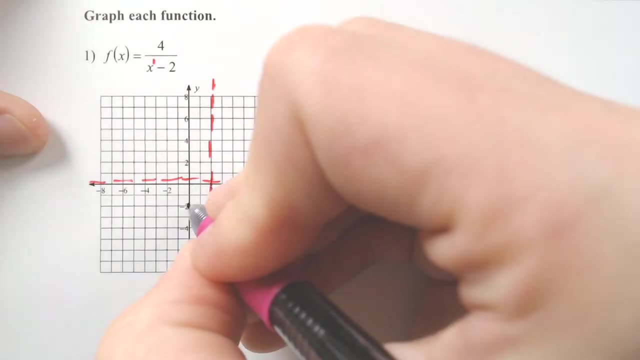 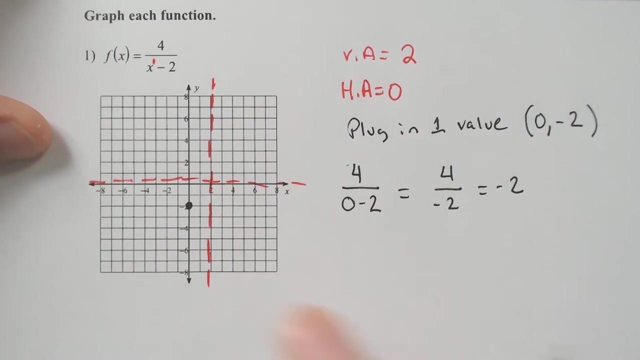 better known as negative two. four divided by negative two is negative two. So we plugged in the point zero and it spit out the value negative two. So that means that there is a dot here at zero comma negative two And that when you only have a single vertical asymptote and a horizontal 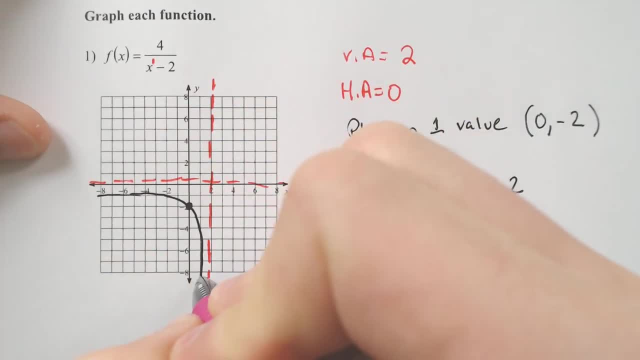 asymptote pretty much guarantees that you have a single vertical asymptote. So that means that this graph is going to look something like this, Where you have it hugging the asymptotes on the left bottom right corner and hugging the asymptotes on the top right corner. OK, Not much is going to. 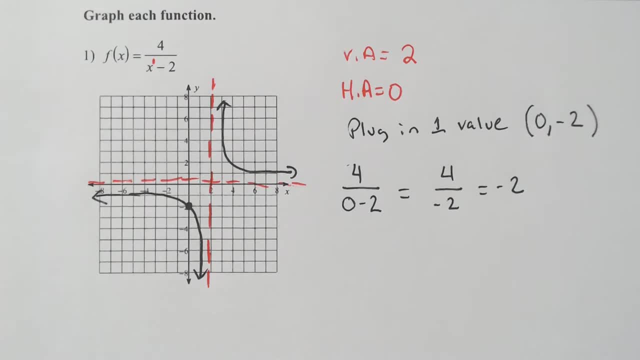 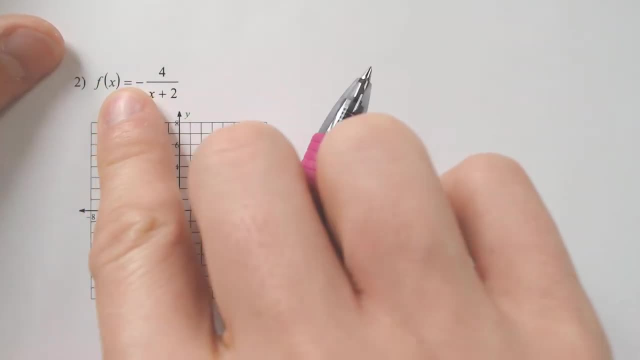 change from that, But there are a lot of other tiny variances that we have to go over. The next variance is this problem, where it's almost the same thing but you notice there's a negative in front and that might change a few things, but not as much as it should. So we're going to plug in. 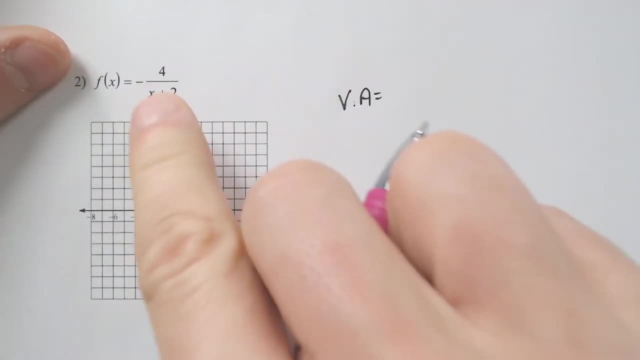 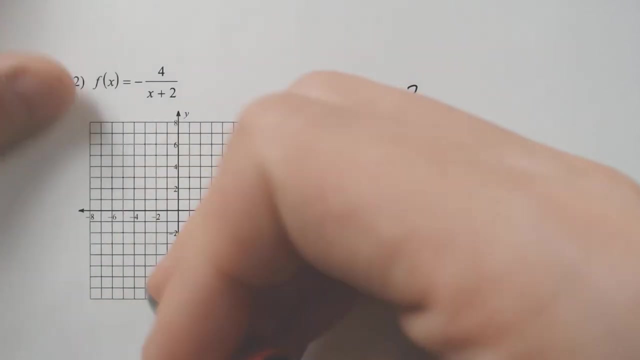 negative two. So we're going to plug in negative two. So we're going to plug in negative two. So our vertical asymptote would be negative two because X plus two you would change the sign. You would get negative two, Drawing it on the negative two. 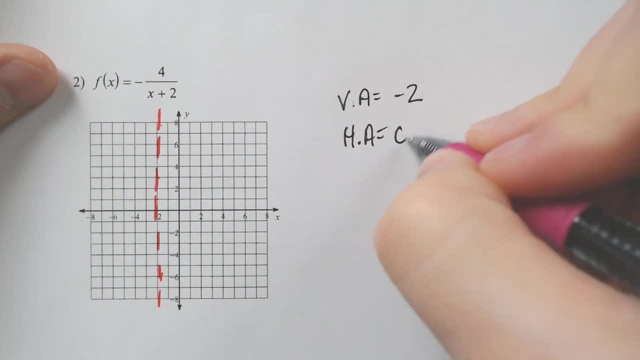 And then our horizontal asymptote again is going to be zero because we have a smaller exponent over a bigger exponent. If you're wondering where I got all these properties from, I got a whole video on how to know what the vertical is and what the horizontal is. 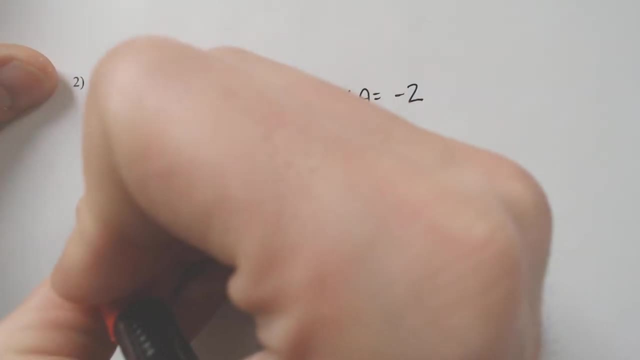 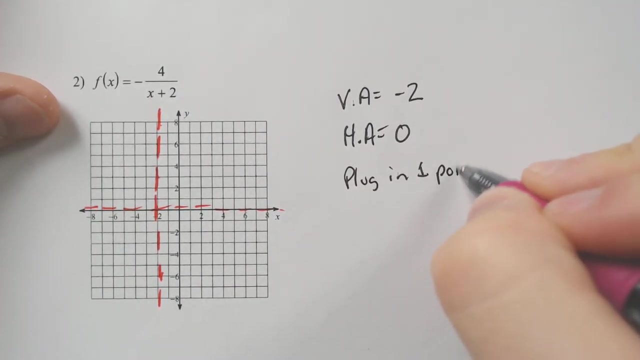 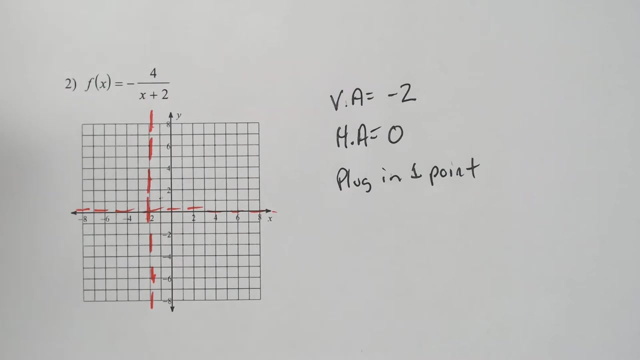 From here We can draw the horizontal at zero And we plug in that one point. So if we plug in one point again, I'm going to plug in the number zero because- why not- it's the Y intercept that tends to be an important point. So if I plug in zero four, zero plus two, I end up with negative four over two again, which happens to be negative two. 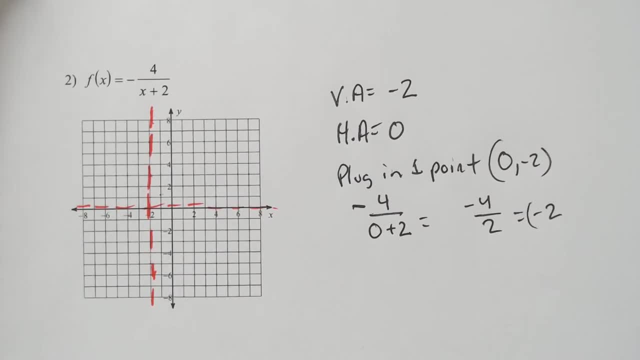 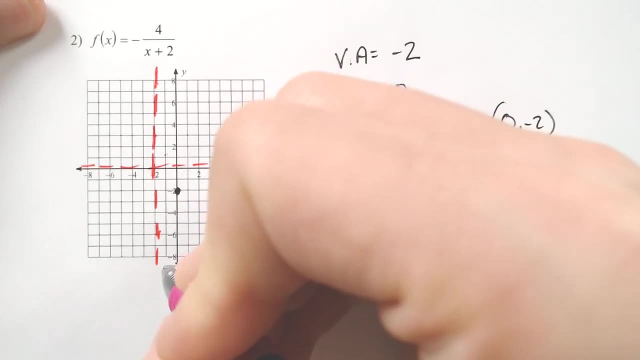 we got negative two Again. that's just pure coincidence, or maybe the fact that I kind of just toggled the first question around a little bit. So from here we're going to plot that point. but look at this time, Instead of it being in the bottom left-hand corner like it was up here, 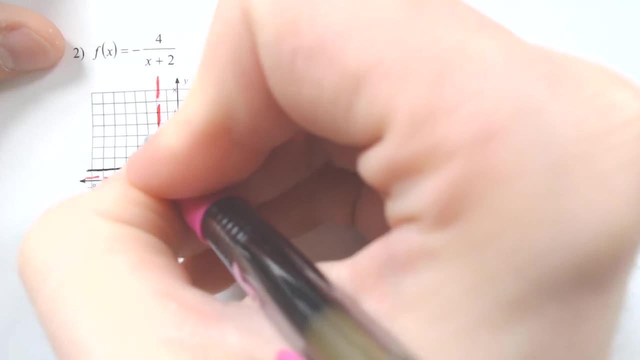 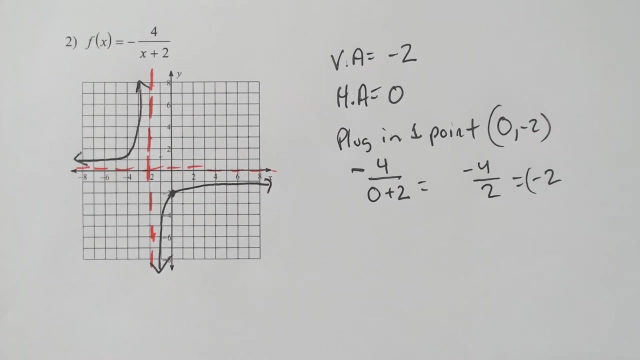 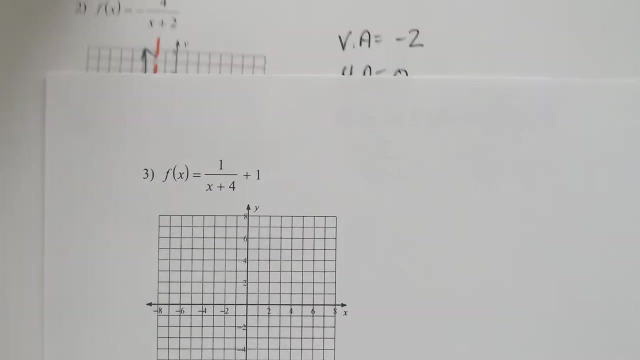 it's in the bottom right-hand corner and it would look more like this: Okay, So the next question we're going to do is going to be very similar to this, but it's going to shift up or down. I think I'm just going to pick the one that shifts up by one. 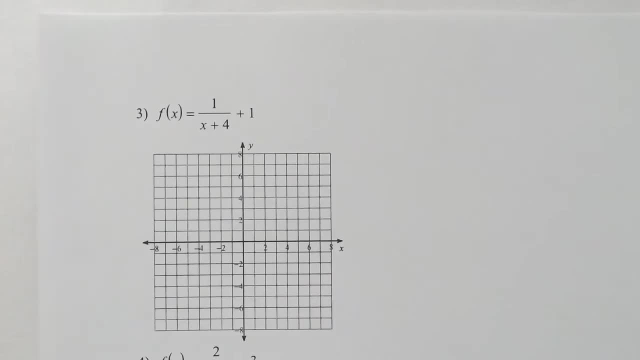 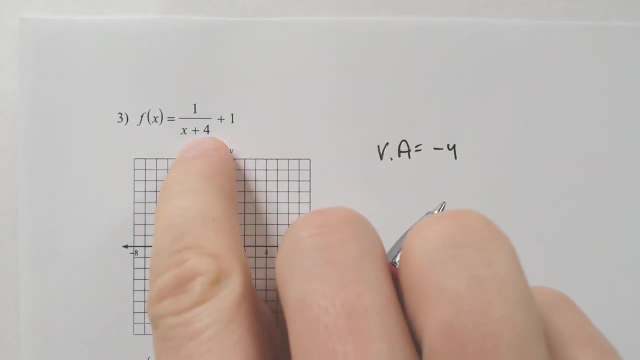 because that will affect the problem so ever slightly. So if you had a problem like this, you still start the same way where you get your vertical asymptote, by changing the sign on the bottom. here, Your horizontal asymptote would have been zero. zero over, one smaller over. 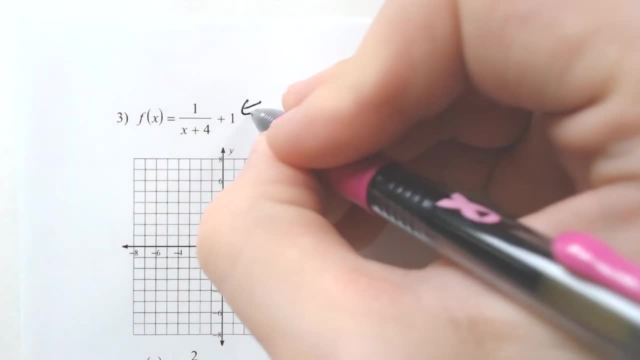 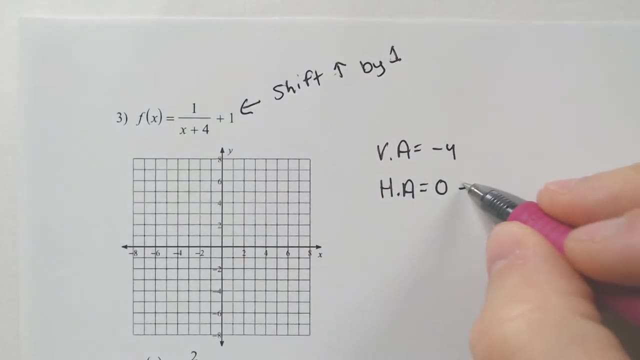 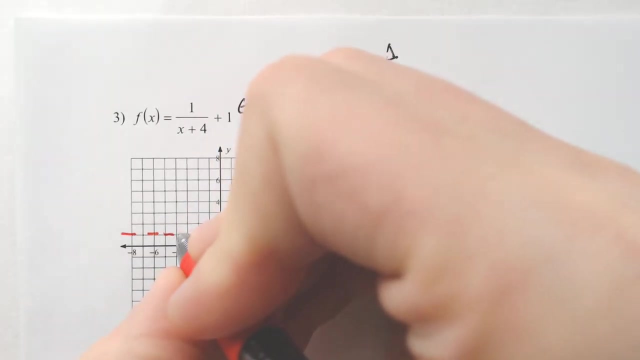 bigger, But because this guy right here, it shifts the entire graph up by one, So this horizontal asymptote is going to be increased by one, leaving me with, now, a horizontal asymptote not at zero anymore, but at one. Now, this would happen anytime you have a. 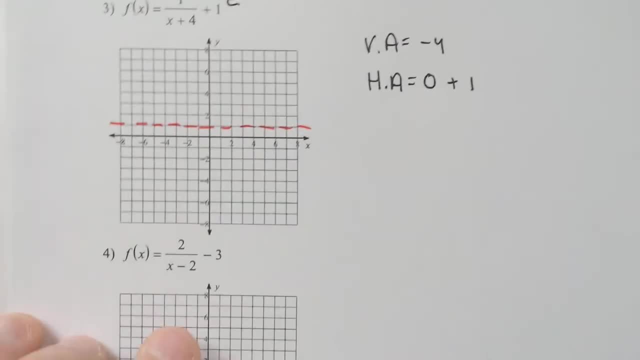 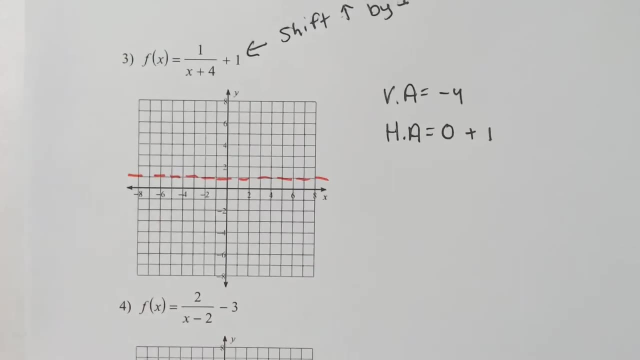 number off to the right. So this one got shifted up by one. This one right here would get shifted down by three. So instead of it having a horizontal asymptote of zero, it would have a horizontal asymptote of negative three. It is not guaranteed to be the horizontal asymptote. 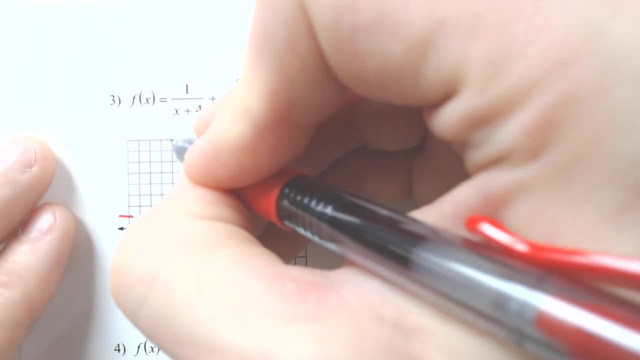 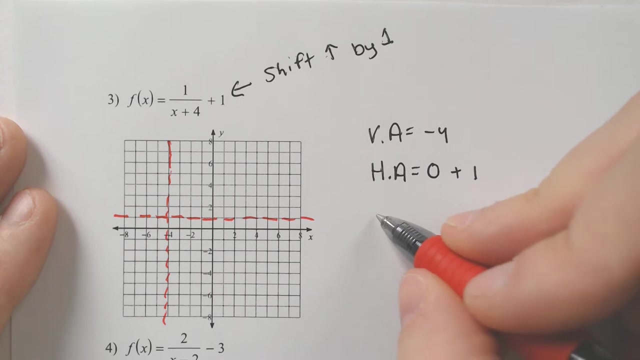 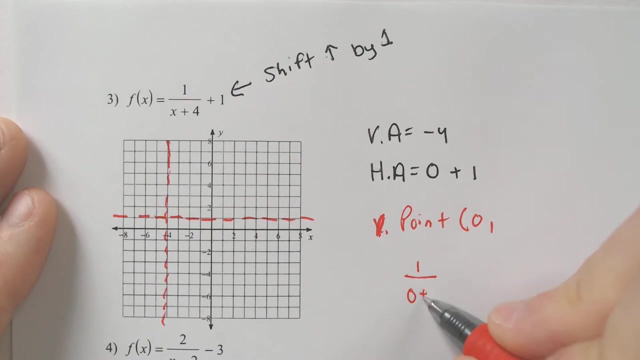 although most of the time it is All right vertical at negative four. Plug in one point. I am again going to plug in zero, but it's probably not the best choice this time. The point: If I plug in zero I would have one over zero plus four plus one, And that would 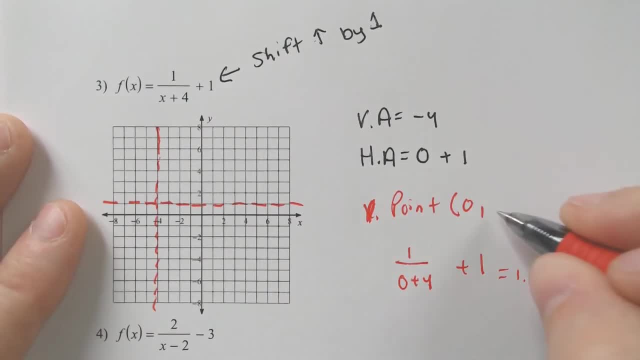 be one fourth plus one, which is 1.25.. It doesn't have to be perfect, because the main thing you're looking for is: are you above or below zero? And if you're above or below zero, you're going to. 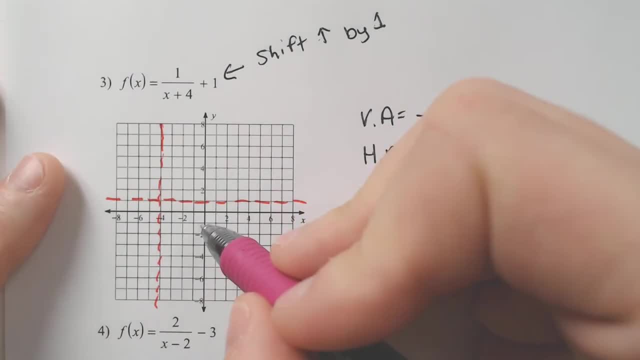 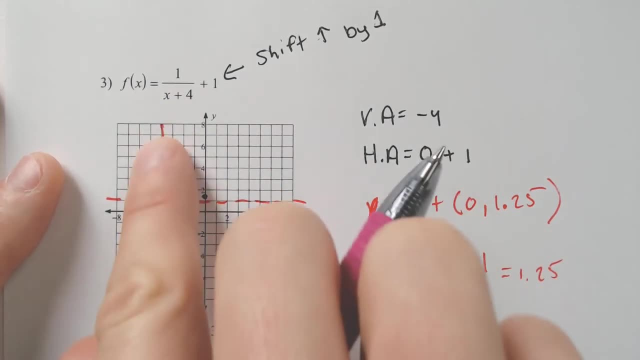 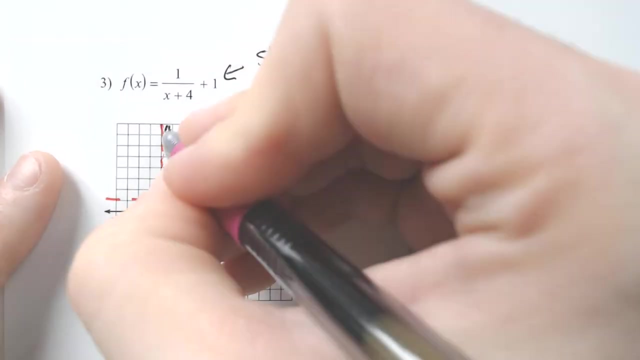 be below the horizontal asymptote at zero 1.25.. I would just barely be above it, And that's why you should really try and aim for something that is near the vertical asymptote when you're plugging in a point, because other times you're guaranteed to pretty much get a decimal Hug the asymptotes. 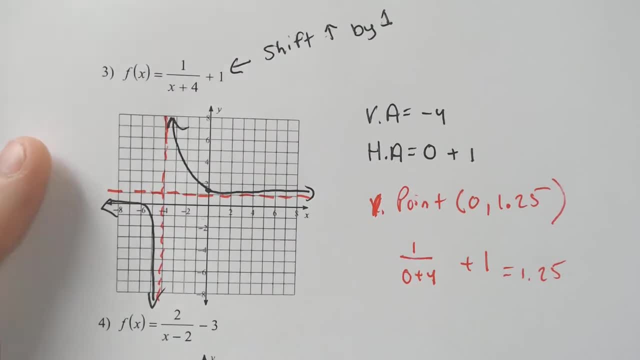 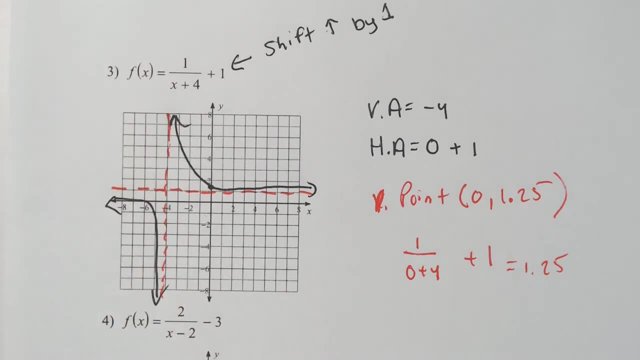 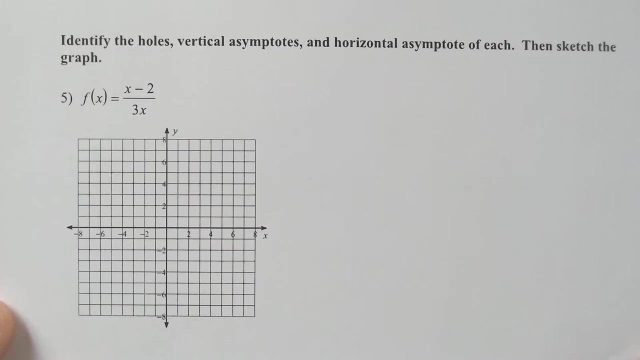 don't go through them and you get the mirror image on the other side. All right, so let's change it up slightly Again. this time we are going to have a horizontal asymptote that is not going to be zero. Okay, so this time we still start with our vertical asymptote. Vertical asymptote. 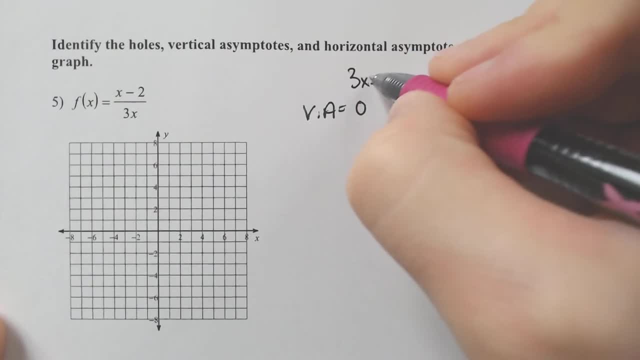 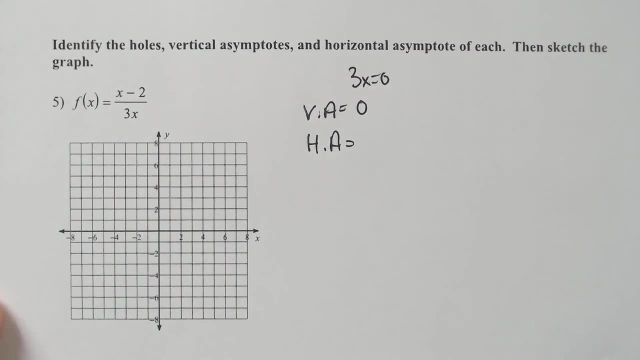 in this case would be zero, because if you were to set 3x equal to zero, you get zero. Our horizontal asymptote this time is a little ridiculous, which is why you have to know the rules. You can't rely on your graphing calculator to tell you everything. It's going to be one over. 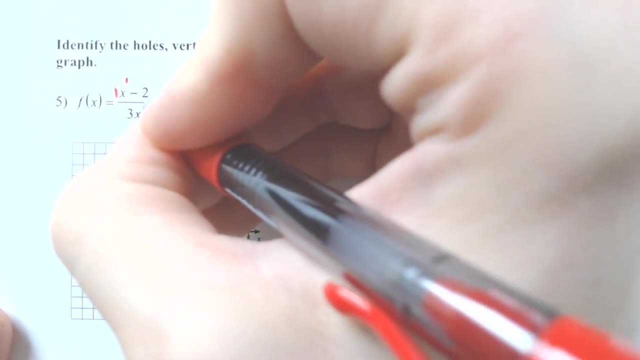 three times zero. So if you were to set 3x equal to zero, you get zero. Our horizontal asymptote this time is going to be one over three, because we have the same exponent over the same exponent, which means the horizontal asymptote is going to be those leading coefficients, one over three. 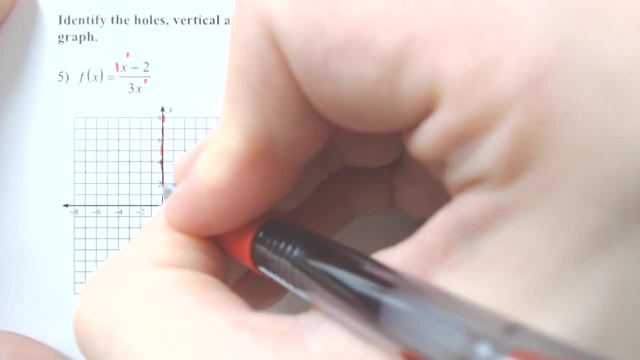 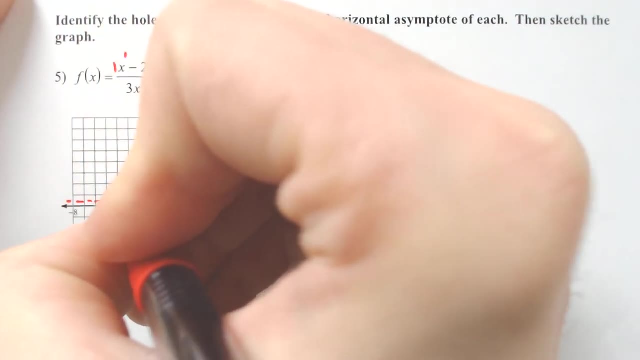 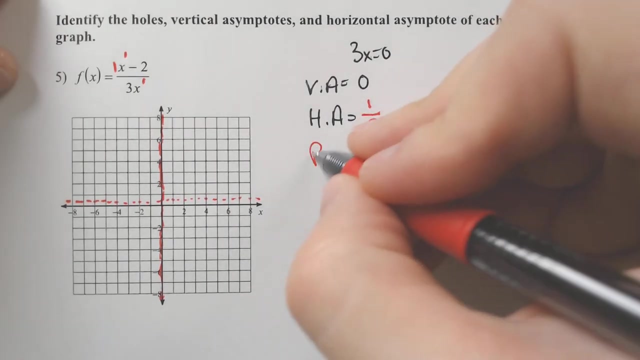 Okay, so vertical at zero, that would be right here. Horizontal asymptote at one third. so that's like just barely above zero. If you didn't know any better, you would probably assume it's at zero. We still have to plug in a point. 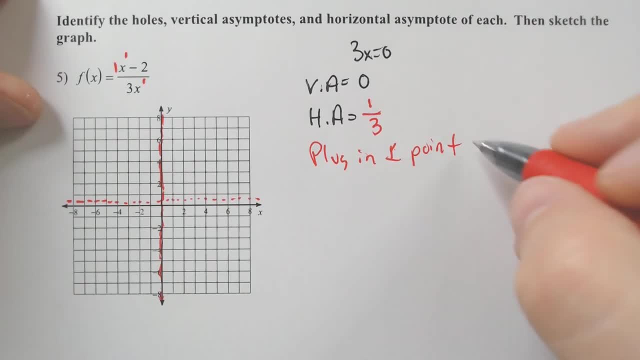 If we plug in one point, I would plug in again the number zero. but I can't. If I plug in zero it's not going to work. So I got to plug in any other point. I'm going to plug in the number one. 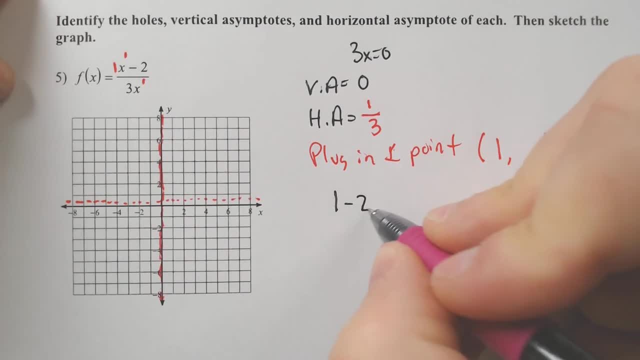 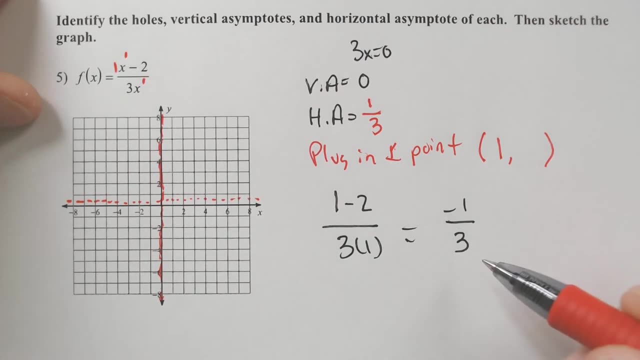 because one is a pretty easy number to plug in. One minus two, three times one, ends up being negative one over three, which is definitely below the asymptote, which is what you're really looking for. Negative one over three is right about here. So if we plug in one point, I would plug in one. 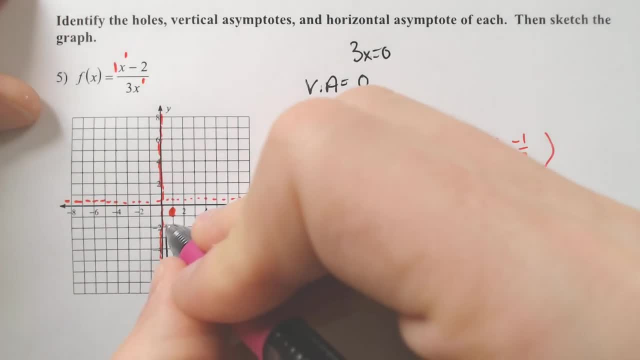 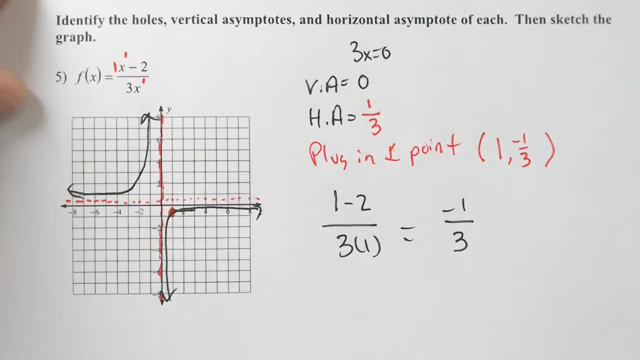 here. So that is below our horizontal asymptote, So that tells me where I am going to be in, like the top right or the bottom left or something like that. So I got my two lines, and the other thing that it's asking us to do here is identify any holes. We haven't done that yet. That's a completely 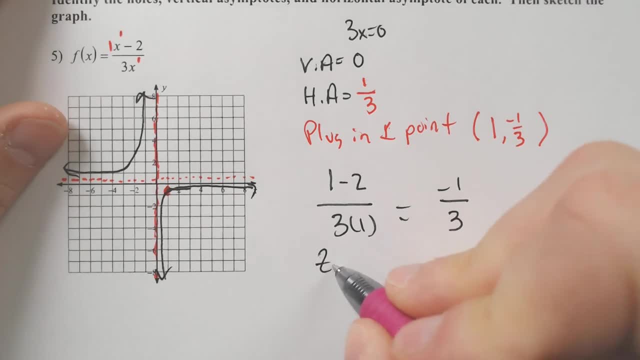 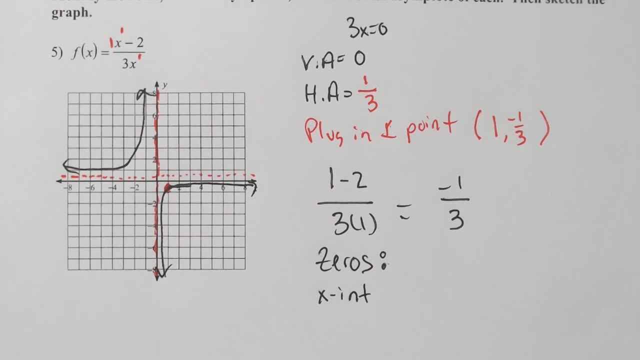 other video Sketch the graph. but sometimes you're asked to find the zeros. The zeros, or the x-intercepts, more importantly, would be found by setting the top equal to zero. So the top equal to zero is how you find the zeros. So 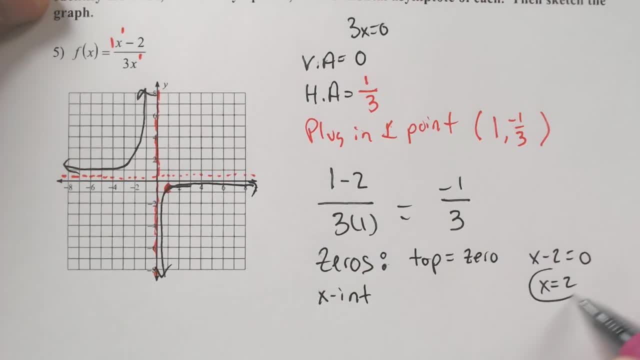 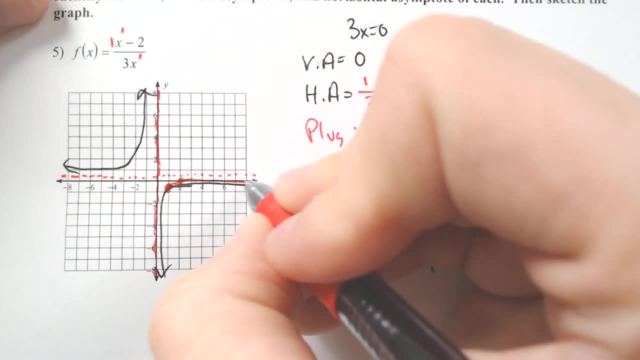 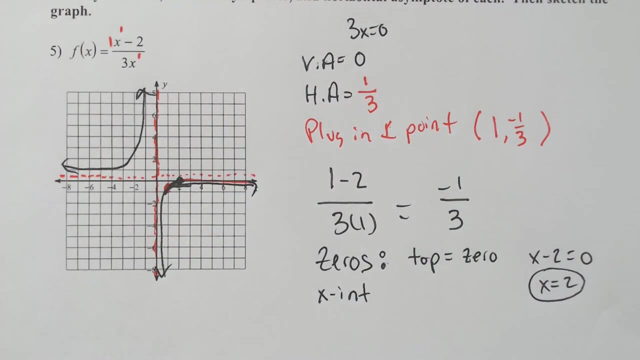 that would mean x minus two equals zero and x would equal two. So I didn't do a perfect job graphing, because apparently we have a zero at two. So it should have crossed that x-axis at two and that is another way that you can confirm how this graph is going to look. But you can only 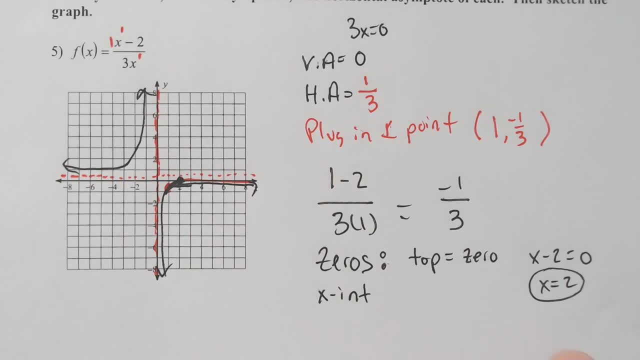 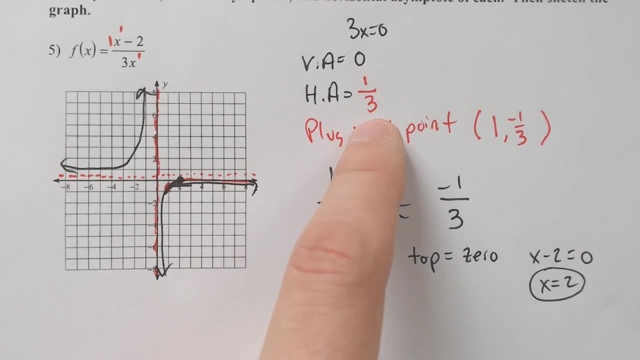 have a zero when the horizontal asymptote's not zero. So this is why sometimes a lot of teachers don't teach the zeros, because sometimes it gets confusing. You can only have a zero when your horizontal asymptote isn't on the x-axis. You can only have an x-intercept when your horizontal 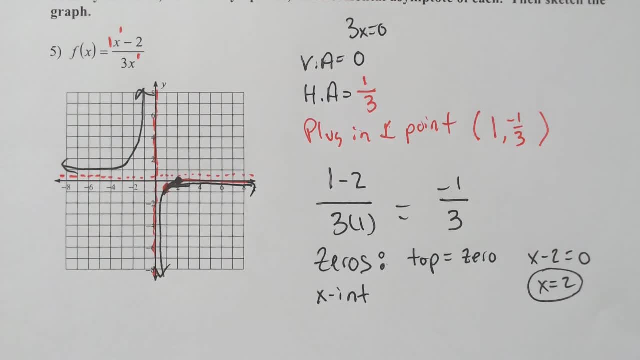 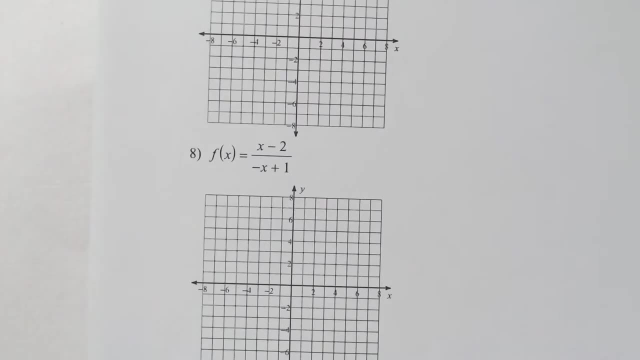 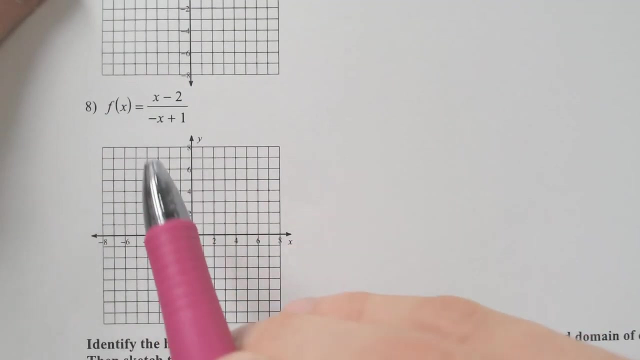 asymptote isn't the x-intercept. Okay, So we got one more, and only one more. This one is going to be right here, It's going to be number eight. So on this one, we got x minus two over negative, x plus one. So our vertical asymptote for the first time. 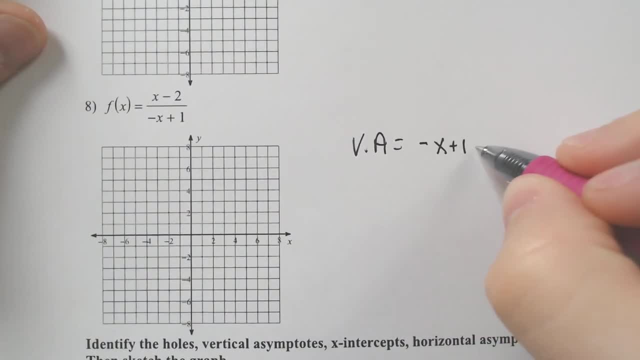 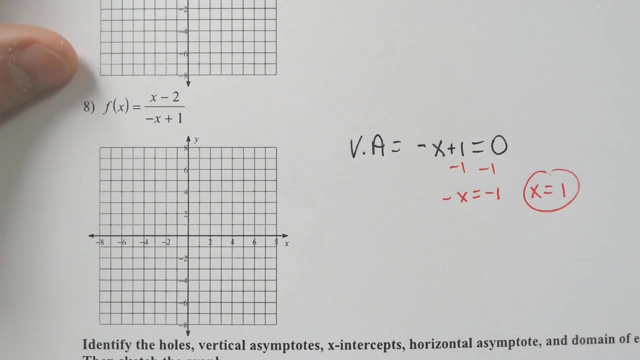 is going to be when you set the bottom actually equal to zero. It's not going to just be change the sign, because if you subtract one you get negative. x equals negative one. which means x equals one is when you actually have the vertical asymptote, when we divide negative one by negative.